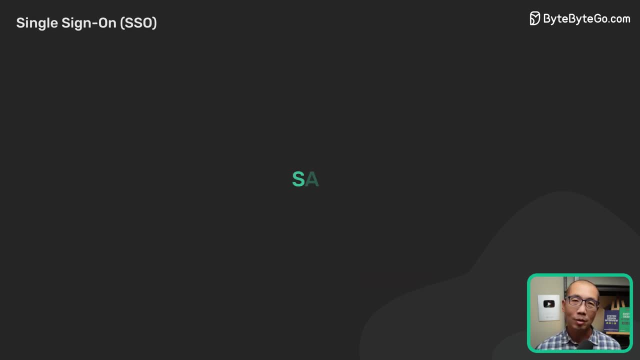 protocols for this authentication process. SAML, or security assertion markup language, is an XML-based open standard for exchanging identity information between services. It is commonly found in the work environment. The other common protocol is OpenID Connect. We should all be familiar with this When we use our personal Google account to sign. 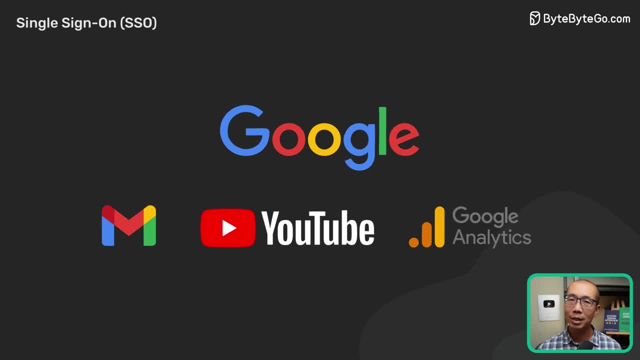 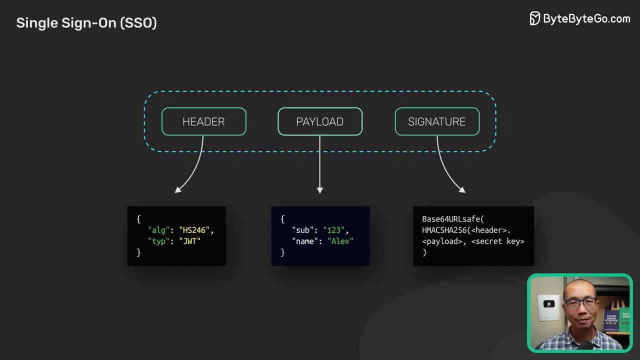 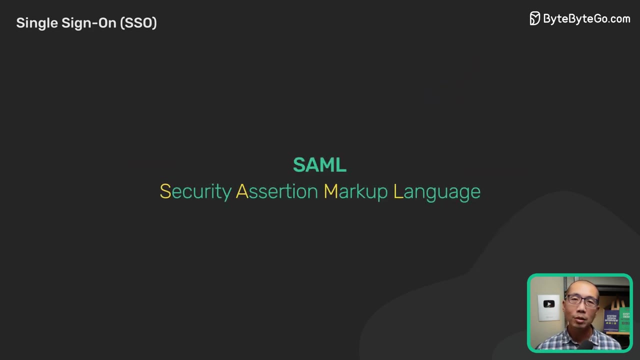 into applications like YouTube. we are using OpenID Connect. It uses JWT or JSON Web Token to share identity information between services. Let's walk through a typical SSO login flow and learn how it works. In this walkthrough, we will focus on SAML. 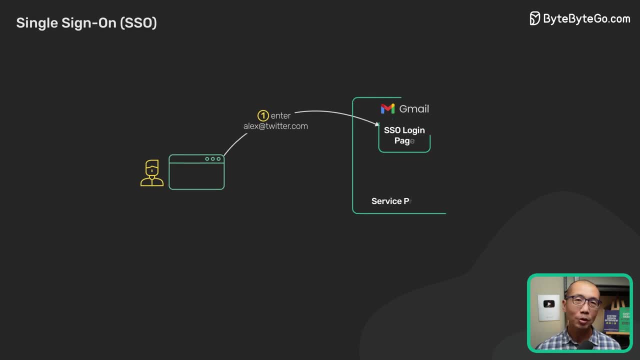 An office worker visits an application like Gmail. In SAML terms, Gmail in this example is a service provider. The Gmail server detects that the user is from a work domain and returns a SAML authentication request back to the browser. The browser redirects the user to. 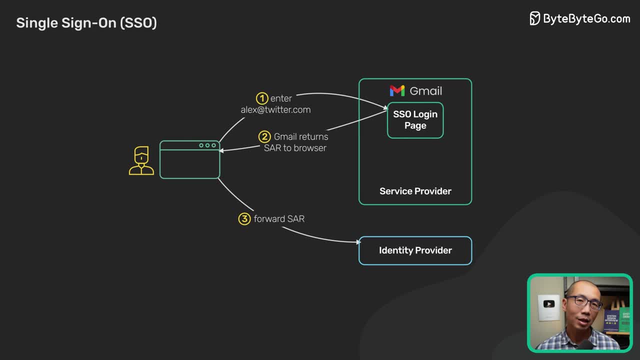 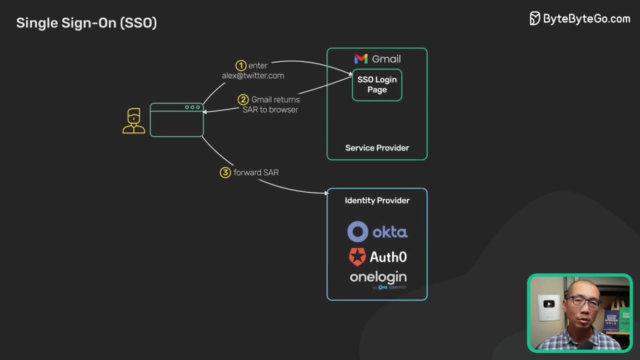 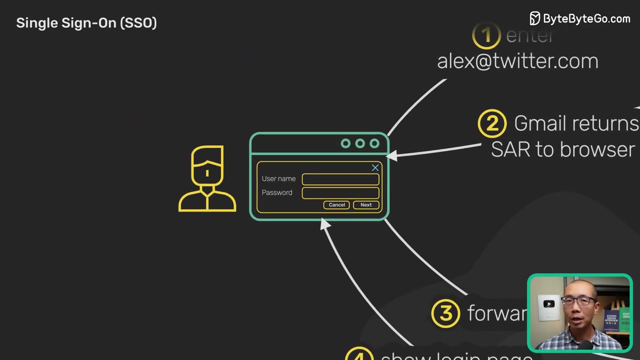 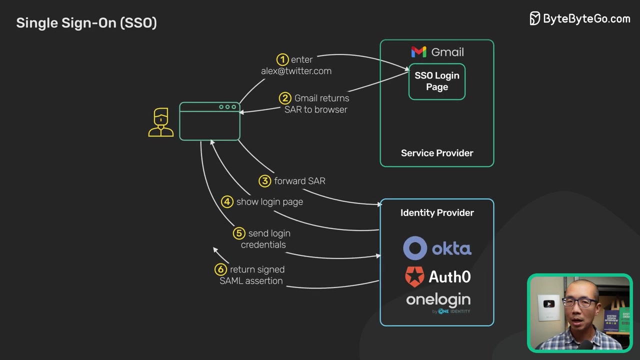 the identity provider for the company specified in the SAML authentication request. Okta call 0 and 1 login are some common examples of commercial identity providers. The identity provider shows the login page where the user enters the login credentials. Once the user is authenticated, the identity provider generates a SAML response and returns. 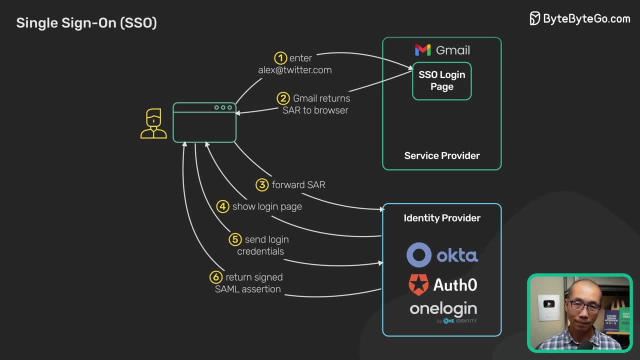 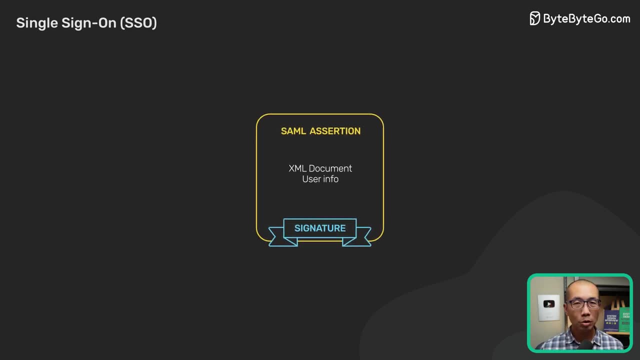 that to the browser. This is called a SAML assertion. The SAML assertion is a cryptographically signed XML document that contains information about the user and what the user is doing. Thisハs our first look into SAML and what the user can access with the service provider. 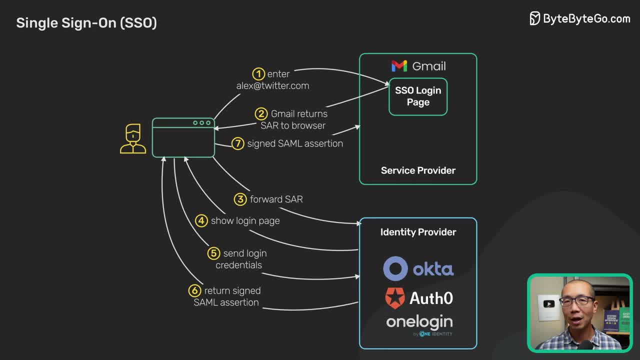 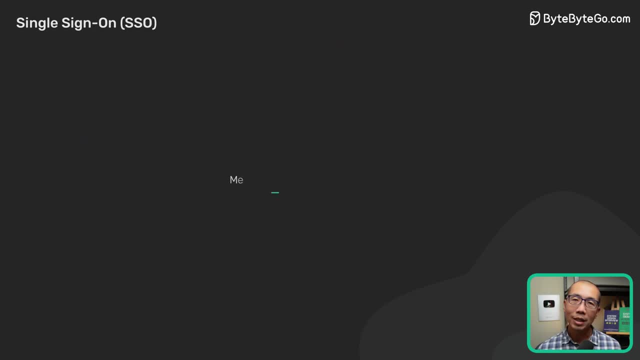 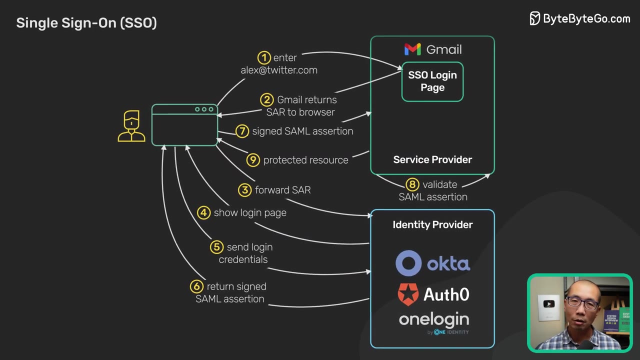 The browser forwards the signed SAML assertion to the service provider. The service provider validates that the assertion was signed by the identity provider. This validation is usually done with public key cryptography. The service provider returns the protected resource to the browser based on what the user is allowed to access, as specified in the SAML assertion. 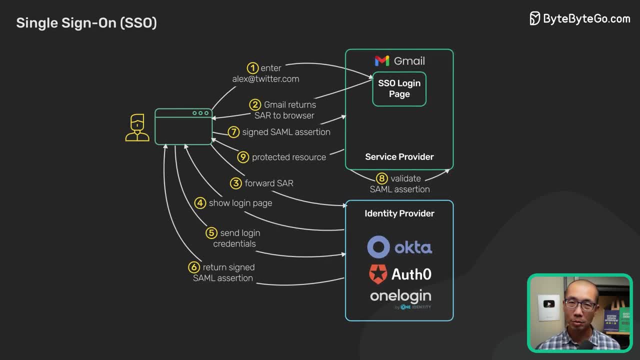 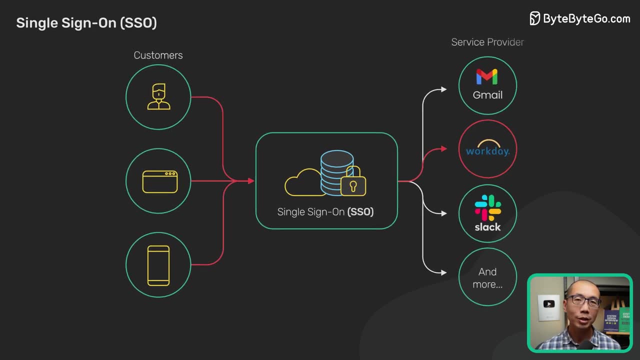 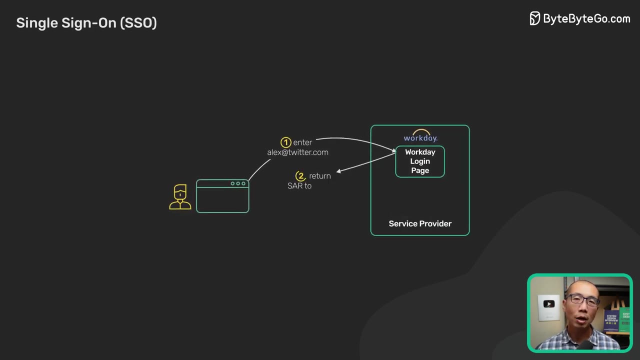 This completes the walkthrough of a basic SSO login flow. Now let's see what happens when the user navigates to another SSO integrated application, say Workday, The Workday server, as in the previous example with Gmail, detects the work domain and sends a SAML authentication request back to the browser.